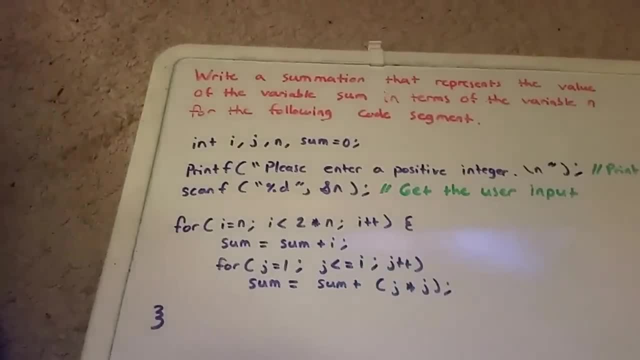 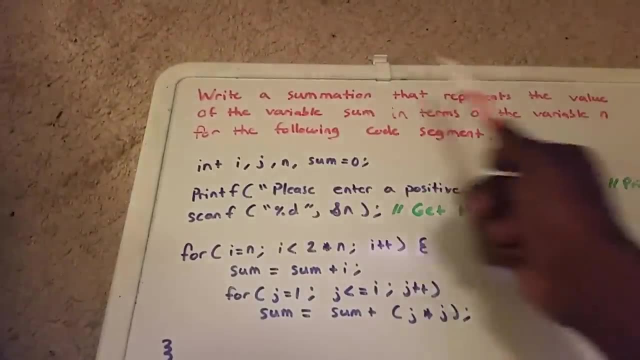 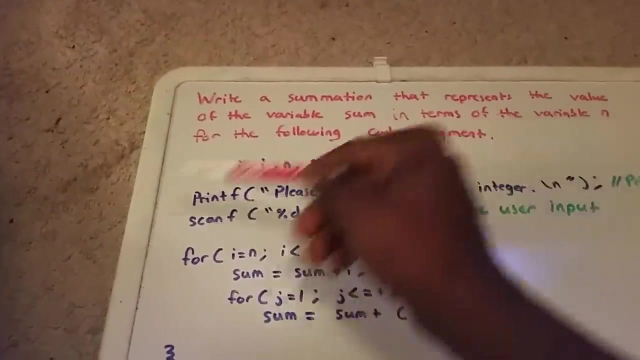 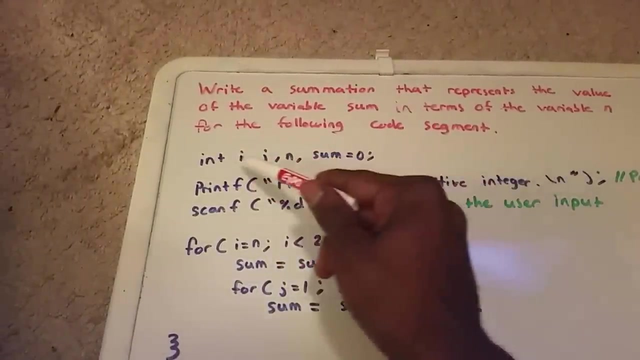 Hey guys, this is a video on summations and algorithm analysis. So here we have a problem. We want to write a summation that represents the value of the variable sum in terms of the variable n for the following code segment. So here we have the code segment in blue and we have our integer variables i, j, n and sum. 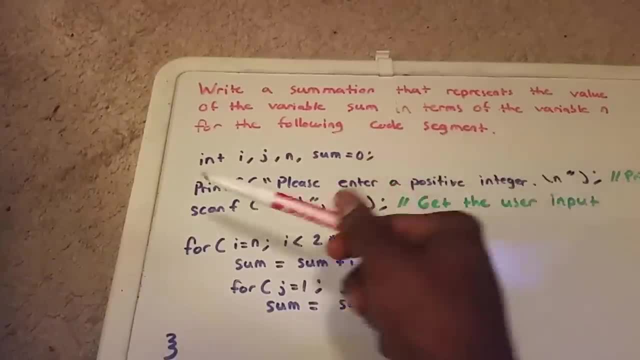 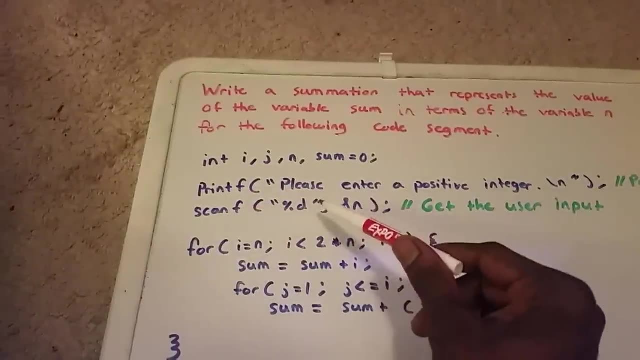 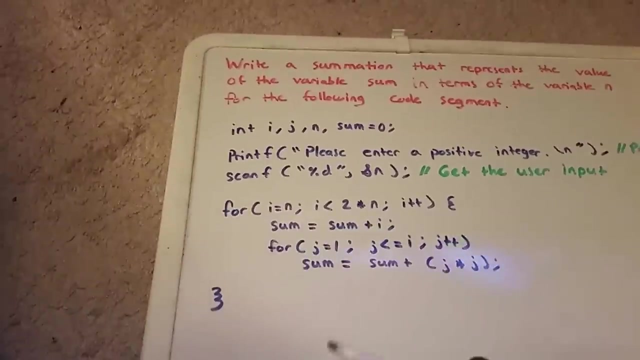 and we set sum equal to 0.. Then we have our print statement It says: please enter a positive integer. and then we get that user input here through the scanf function And then we have two for loops here And within the first for loop it 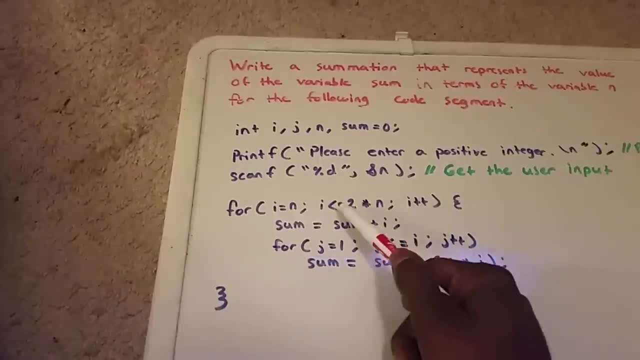 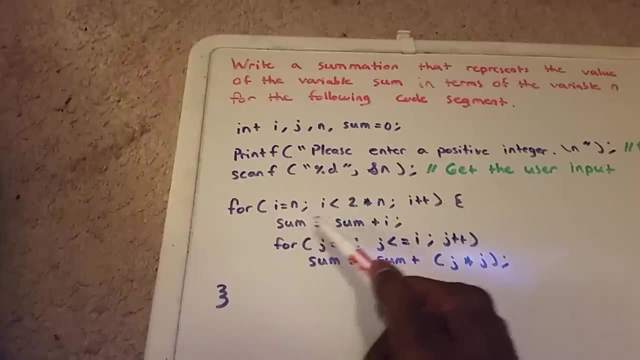 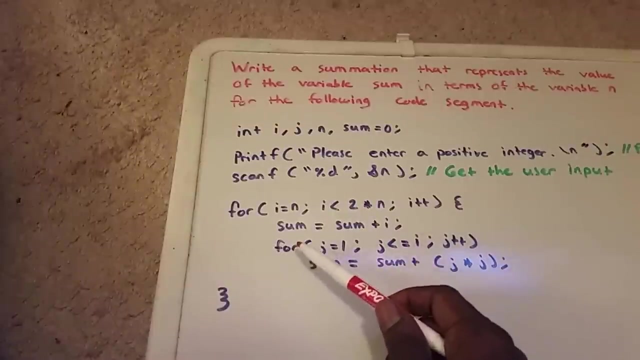 goes from i equaling n to i less than 2 times n, and then i increases by 1 each time And our sum equals sum plus i. And then, within this for loop, we have another for loop, And this for loop goes from j equaling 1 to j less than or equal to i. 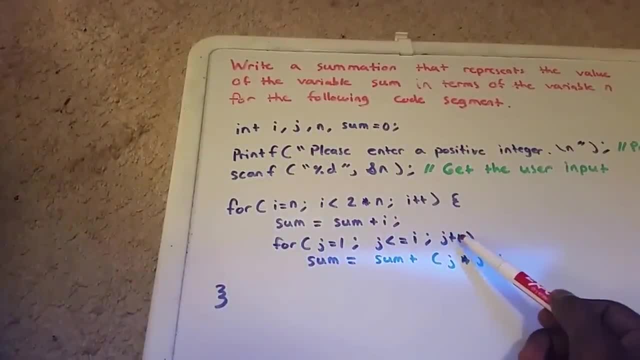 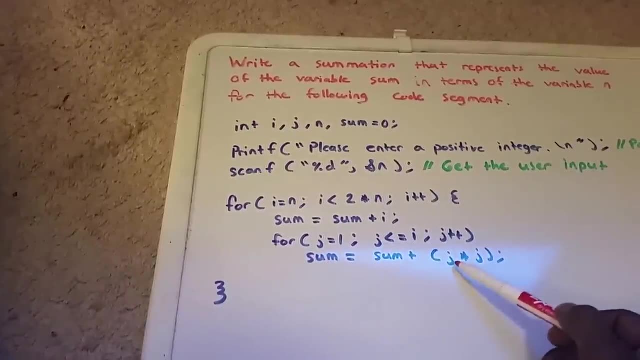 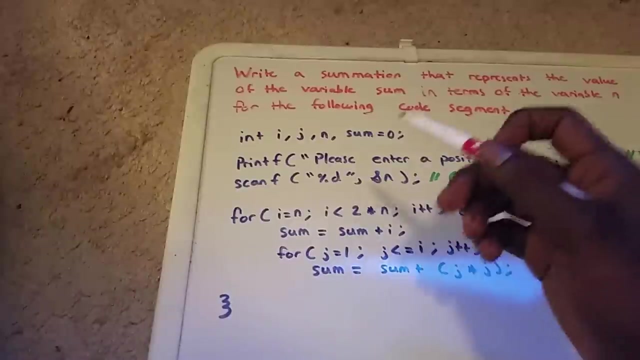 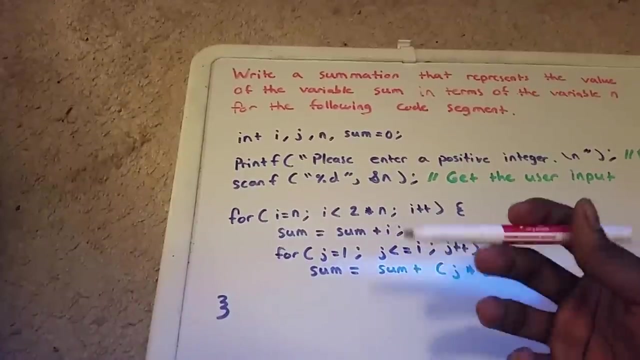 and j increases by 1 each iteration. Then within this for loop here our sum equals sum plus j times j. So this for loop is within this for loop. So now we need to write these for loops here And the sum here as a summation. 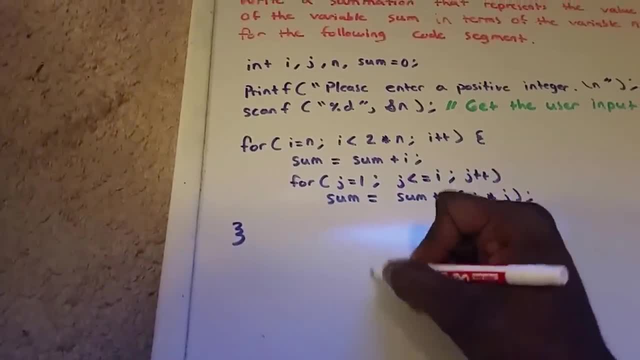 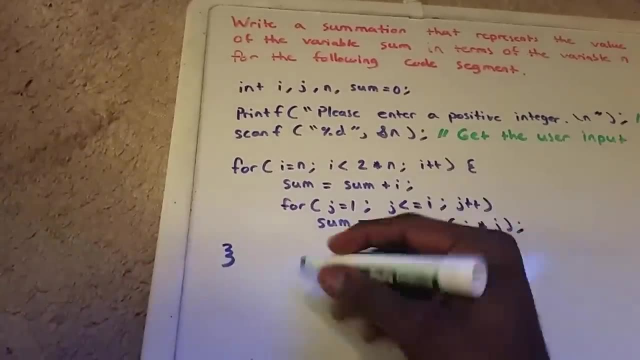 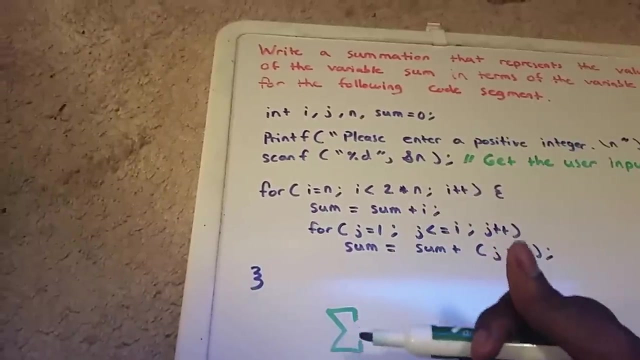 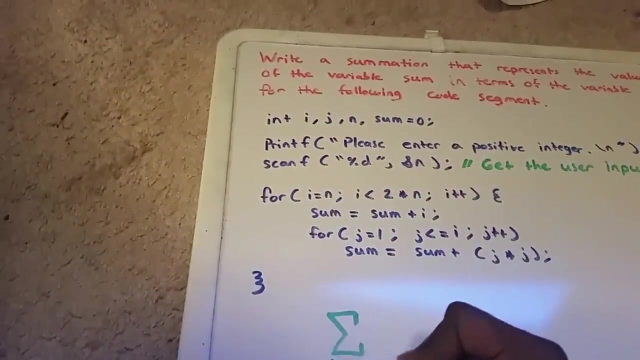 So let's get started. Like my marker has ran out there, I go ahead and use a green marker, So we have a for loop, and the for loop can always be represented by summation. and our first for loop here goes from i equals n, so i equals n, to i less than two times n, so it doesn't go to. 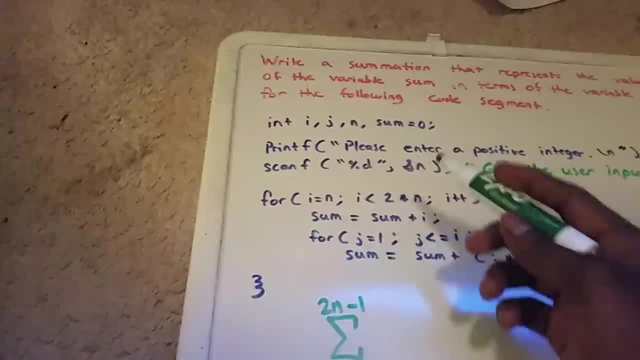 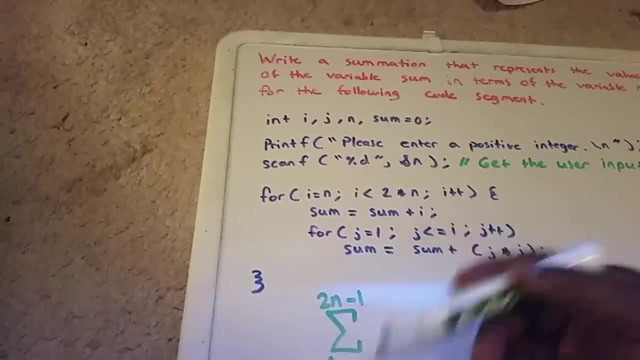 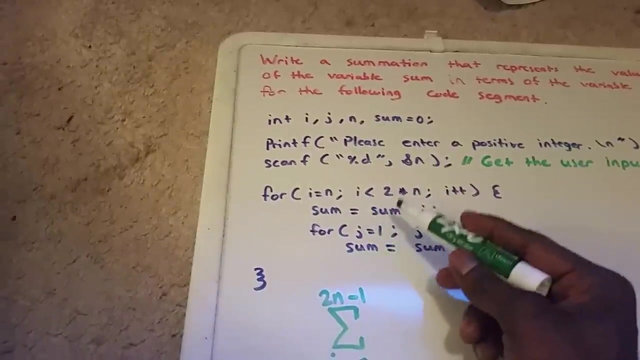 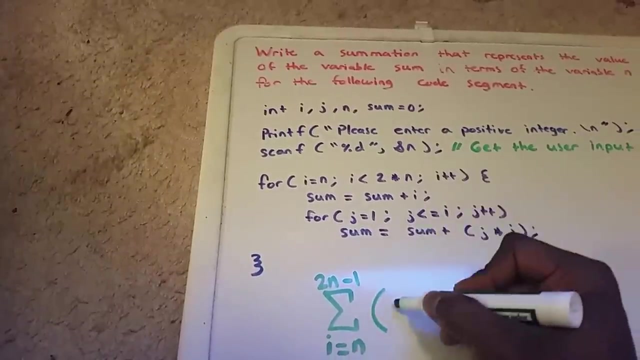 two times n, it goes one less. if this was an equal sign, it would go all the way to two times n. and then i increases by one each time. so that's the iteration. that's great, uh, next we have our sum equaling sum plus i. so, within this loop, here we have our sum equaling sum.